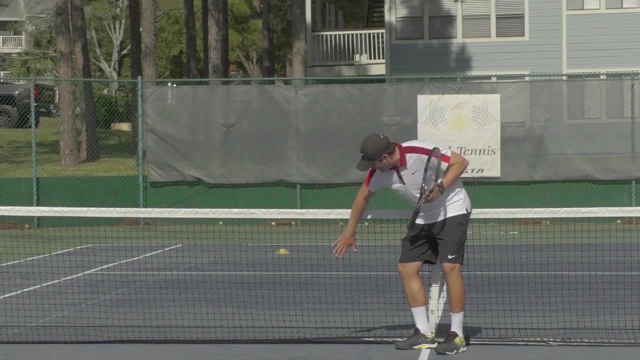 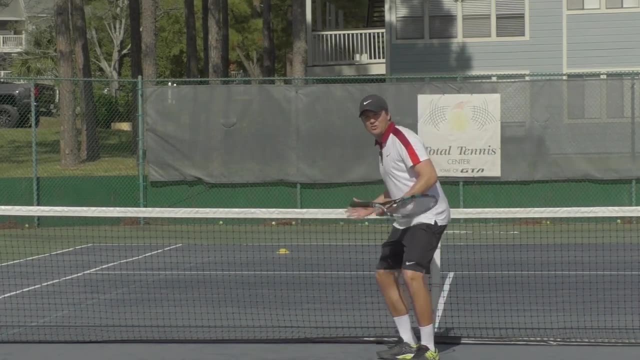 through the net, So you can see that yellow cone through the net over here. So what happens is it tricks people to thinking that they can swing across their body and also they don't have to use their legs. Now, what you want to envision is: you want to envision having 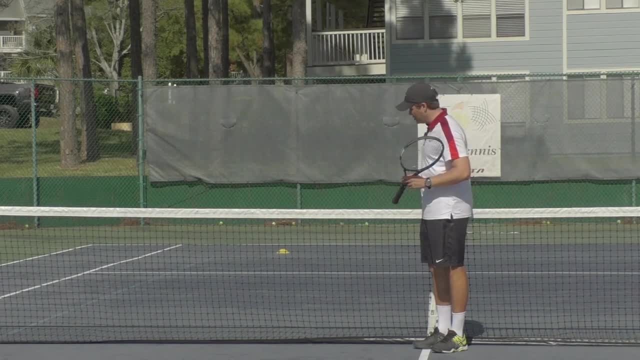 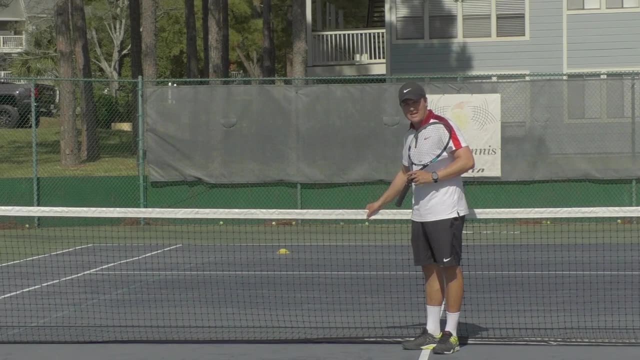 an air target. So one way we can do that I'm going to show you: you can take a sheet or anything that's opaque and lay it across the net so it really blocks the view through the net And that will help you to understand and visualize that you need to have an air. 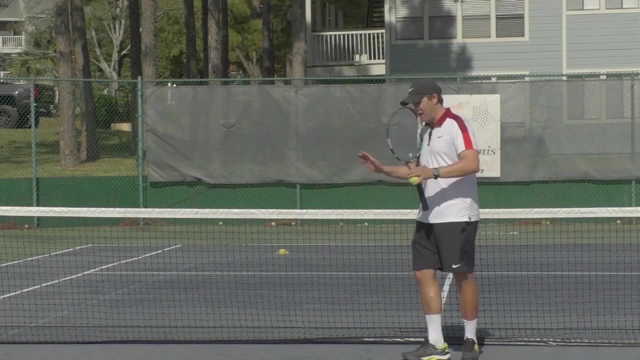 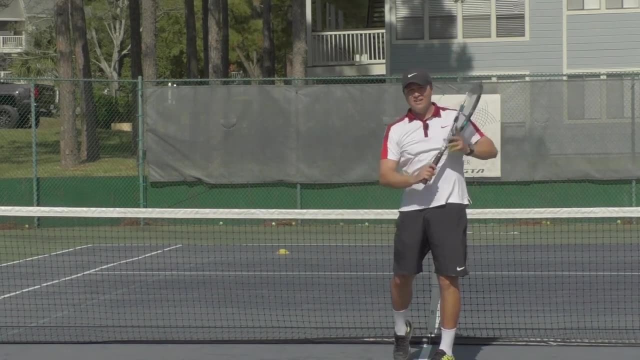 target. But when we do that, we notice that players are then, more naturally, are going to bend their knees, get the racket lower and they're going to swing from more low to high. So when you swing from low to high, you're going to develop topspin, but also 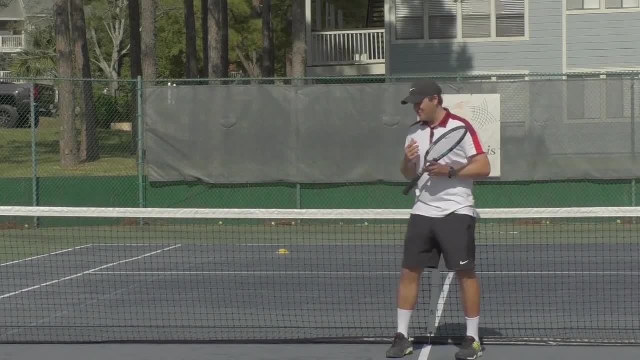 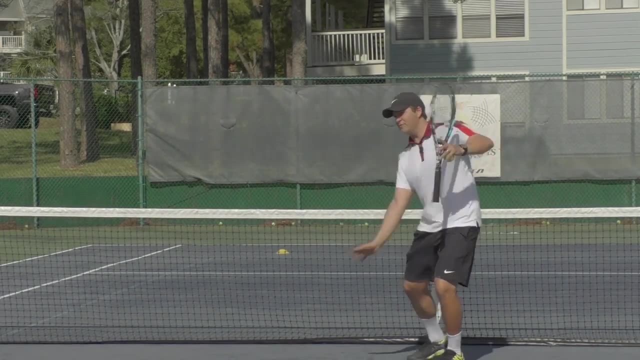 you'll develop a longspin. Let's take a look at the drill in action. I'm going to lay a sheet across the net blocking the view through this net over here, forcing me to get low with the legs and to swing from low to high so I hit good ground strokes with long hitting zones and good topspin. 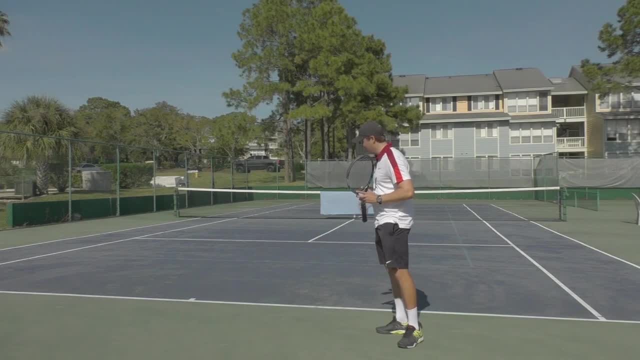 Okay, so, as you can see, I've placed that sheet over the net and now that target, which we saw through the net, is no longer visible And actually, if I'm looking over the net, I don't see any part of the tennis court. All I'm seeing is the backdrop over there. 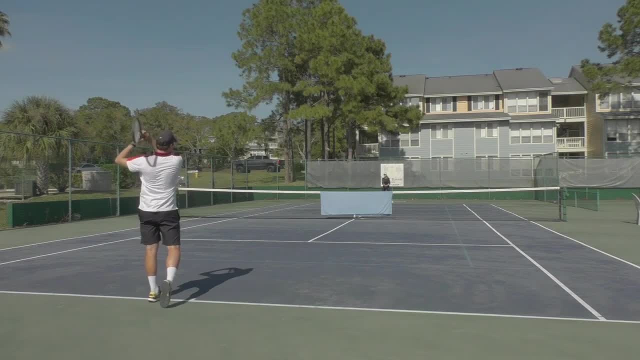 So I'm going to rally here with Ava And now it's going to force me to have that air target where I have to use my legs more and swing from more low to high, because it's going to give me the perception of having to lift the ball rather than have to pull the ball across my body. 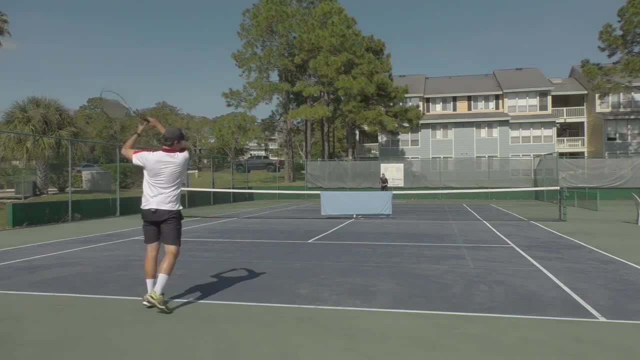 So this is a really good exercise to help you with that And then what you could do. you can progress it from rallying to actually playing points this way. So give the stool a try, Find something to cover the net with and then with the partner. 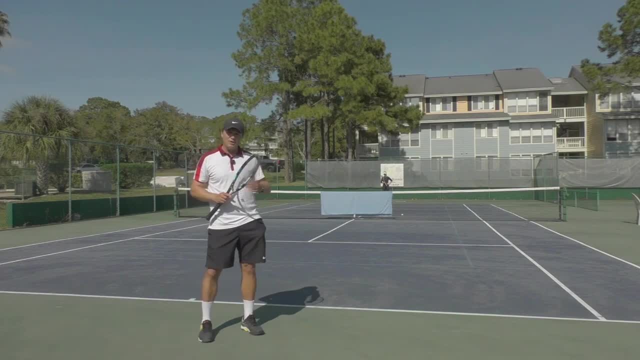 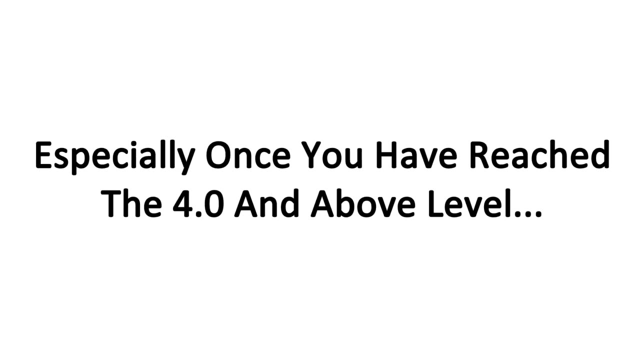 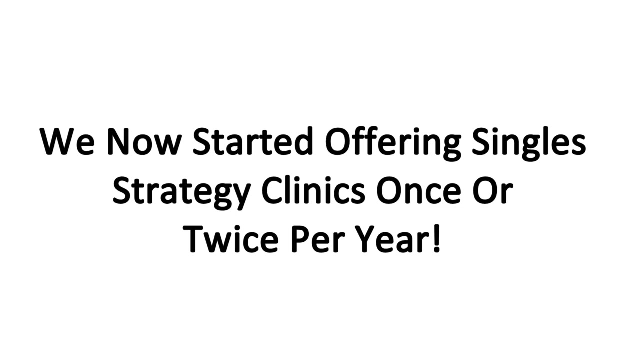 you want to start by rallying and even play some points out. If you like this video, give us a thumbs up and leave your comments below. Thank you, Because single strategy can be so important for your game, especially once you've reached the 4.0 and above level, we now started offering single strategy clinics once or twice per